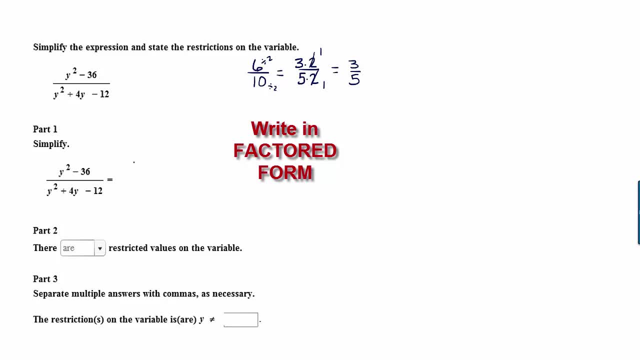 But we actually have it written in factored form: y squared minus 36 fits the pattern of a difference of squares, So it factors into conjugates. Y squared plus 4y minus 12 is a trinomial, The leading coefficient as 1, so all we need to do is look at the negative 12.. 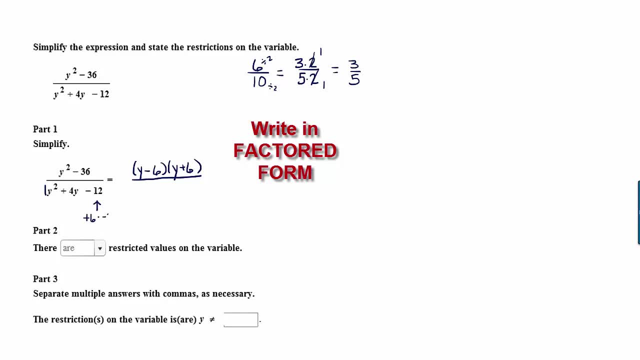 We're looking for factors of negative 12 that add up to 4.. Positive 6 times negative 2 gives us negative 12.. 6 plus negative 2 adds up to positive 4.. This tells us that if we multiplied y plus 6 times y minus 2, by foiling this out, we would get y squared plus 4y minus. 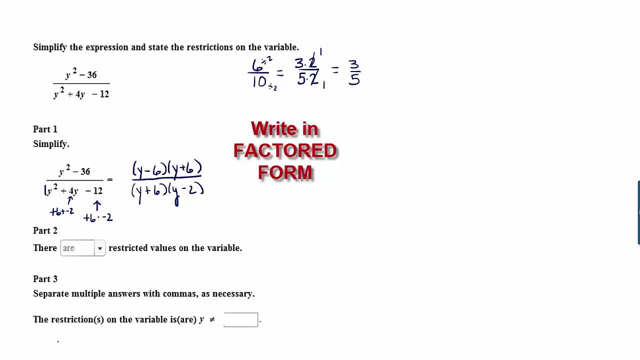 12.. This is the factored form of the rational expression, and we can see that we do have a common factor in the numerator and denominator. we have y plus 6. Dividing those out leaves us with a factor of 1, and so this expression. 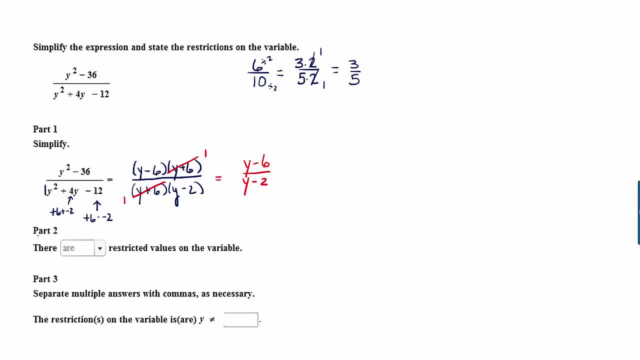 reduces to y minus 6 over y minus 2.. In the second part, they ask whether or not we have restricted values. To have restricted values means that it's possible that the denominator is equal to zero. For example, in this case, in order for y minus 2 to be 0, we would have y equal to 2.. If you were to plug in 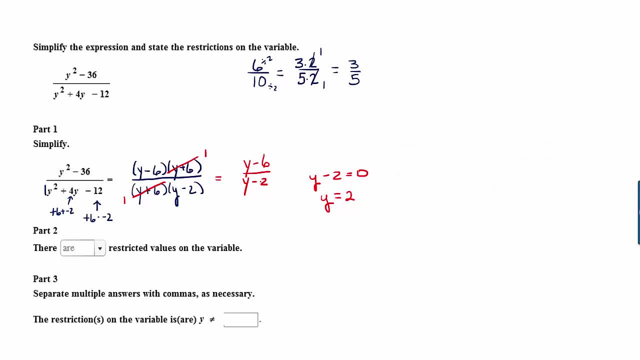 2. in other words, we would get a 0 in the denominator, causing the expression to be undefined. So the answer to part 2 is that yes, there are restricted values. In the second part they ask whether or not we have restricted values To have. 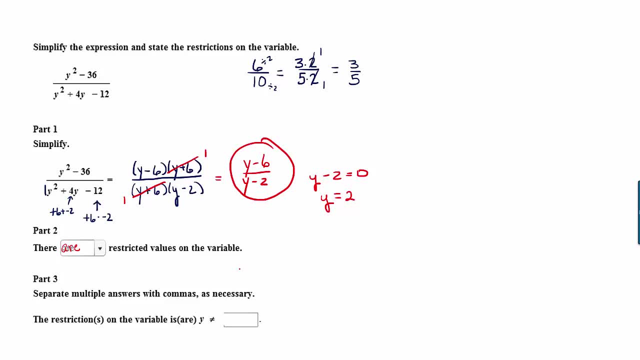 restricted values. But it's not as obvious as just looking at y minus 2.. In fact I kind of exaggerated when I said these two expressions were equal, because when I cancelled out y plus 6, I cancelled out the possibility of having a 0 for this expression. So you always have to go back and look at the 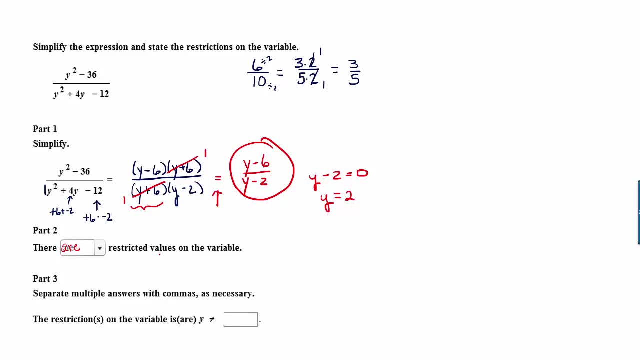 uncancelled version, if you would, if you want to put it that way, of the rational expression for part 3, where it asks you to find the restrictions on the variable. Don't look at this last reduced form of the rational expression, but set the denominator. 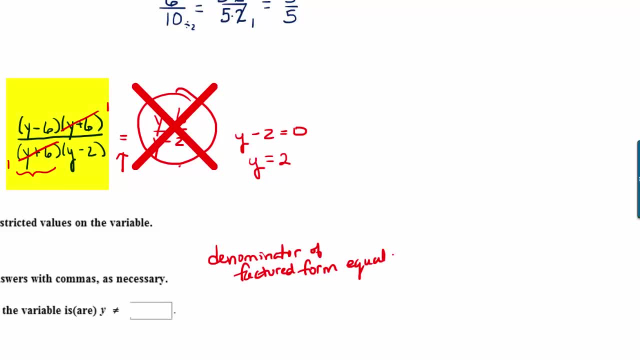 of the factored form equal to 0 and solve for the variable. This guarantees that we get all the restrictions. So y plus 6 times y minus 2 equals 0. can only happen if either y plus 6 is 0 or y minus.